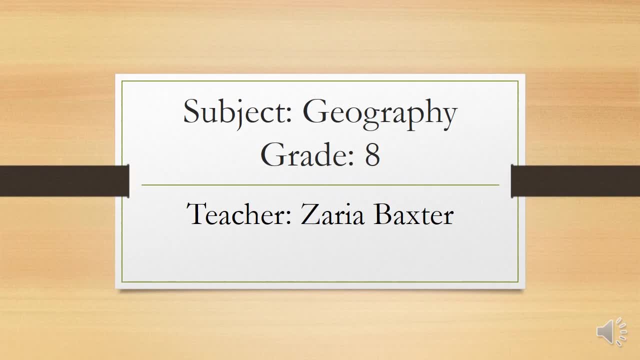 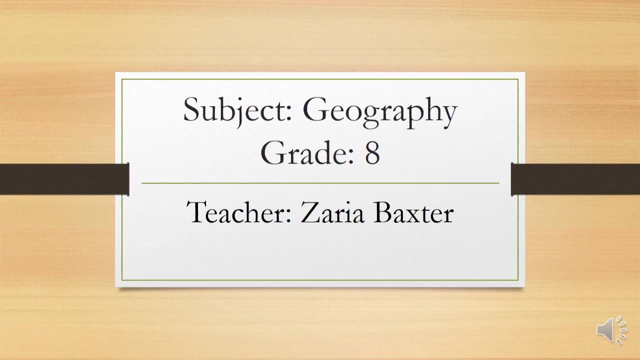 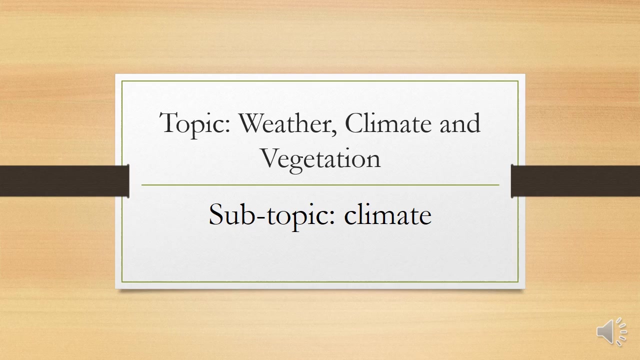 Good day, boys and girls. This is Mrs Baxter, and I'm here to bring to you your lesson for today on weather, climate and vegetation. Weather, climate and vegetation, That's our broad topic, but our subtopic is climate. 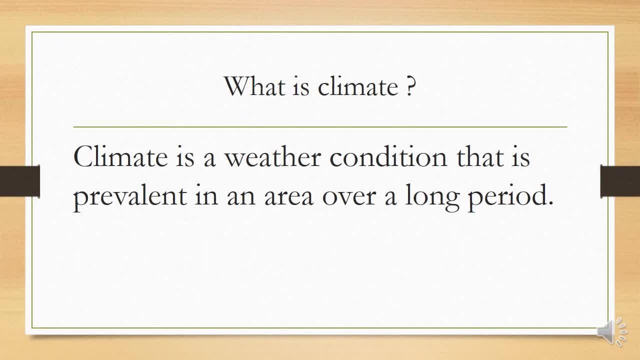 Now, boys and girls, we had distinguished the difference between weather and climate in our previous lessons, and we established that climate is a weather condition that is prevalent in an area over a long period of time, while weather is rarely the day-to-day changes in the atmosphere right. 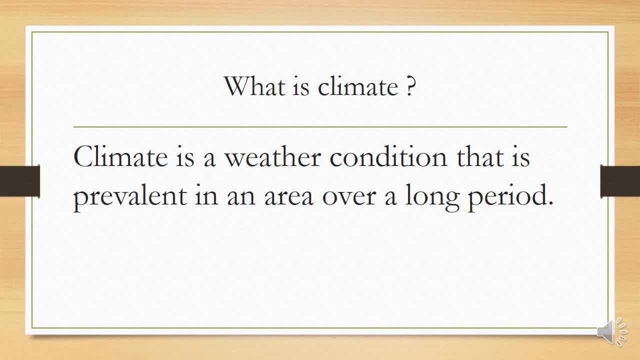 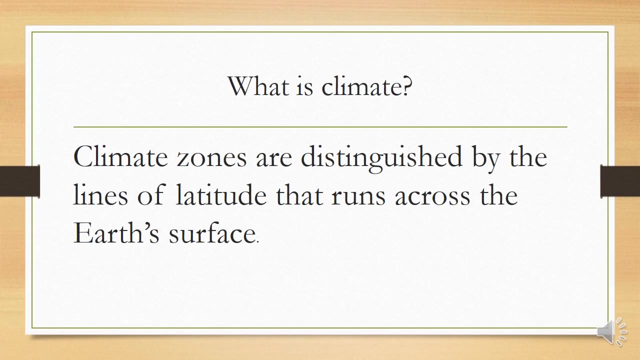 Take first climate. Take second climate, For example, Jamaica. we normally are exposed to sunny conditions and as a result of that, we fall in the tropic zone. We are in the tropics, Students. climate zones are distinguished by the lines of latitude that runs across the Earth's surface. 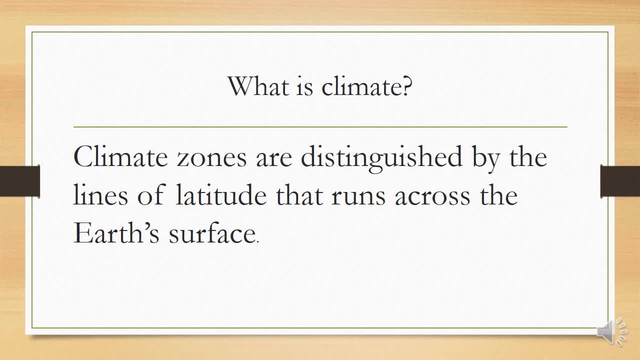 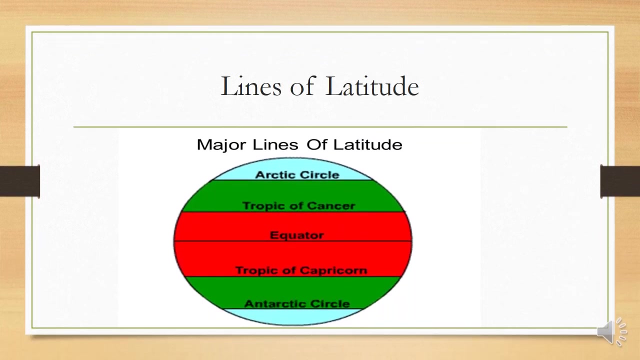 Now you would have learned from even the primary level that lines of latitude are rarely imaginary lines, but of course they are used also as markers to distinguish which countries fall in which climate zone on the Earth's surface. Now, boys and girls, here we have our major lines of latitude: the Arctic Circle, the Tropic of Cancer, the Equator, the Tropic of Capricorn and the Antarctic Circle. 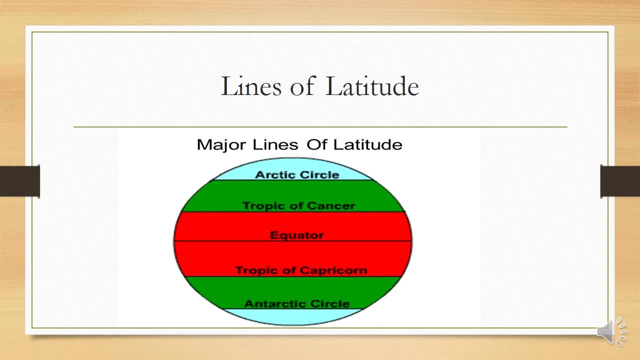 Each area is color-coded. The areas to the north and south in blue represent the polar zone- very cold regions- The areas in green represent the temperate zone and the areas in red represent the torrid zone or the tropics. Here we have a diagram.